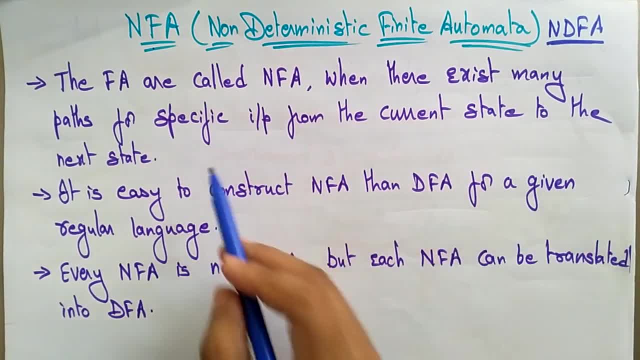 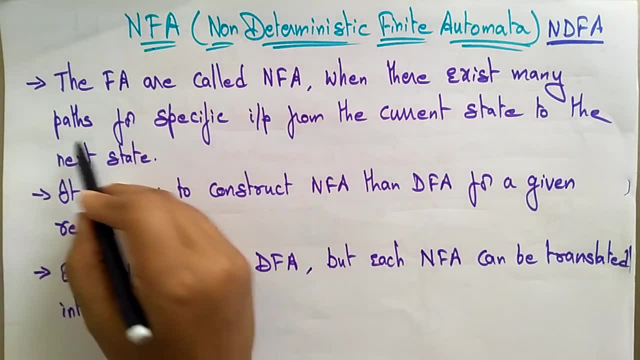 exist many paths for specific input from the current state to the next state. So did you observe the difference between NFA and DFA here? In DFA, there exist only one path for specific input from current state to another state. Suppose if 0 is there, the 0 can go to. 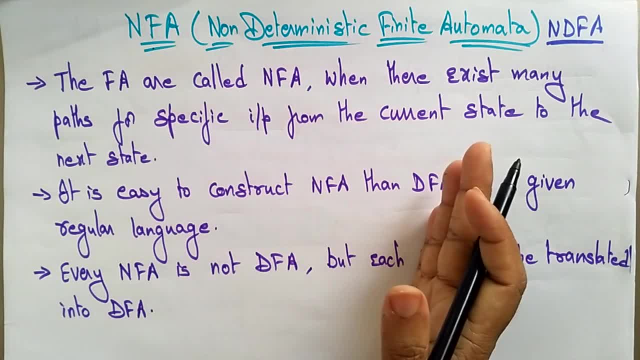 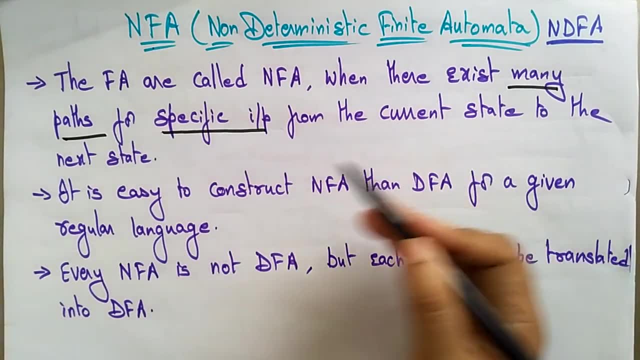 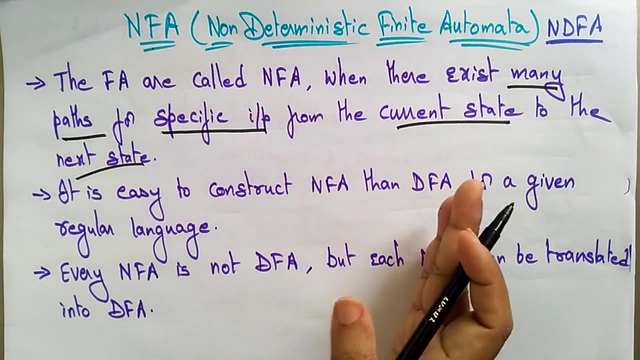 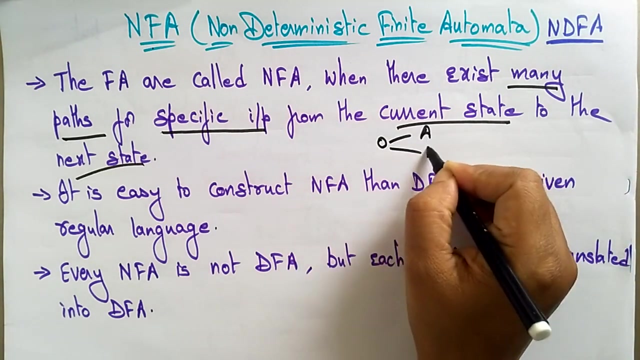 only one state, not twice. But in this NFA there is many specific paths for specific input from the current state to the next state. So many paths for specific input. Suppose 0 is there. the 0 can go to many paths. Either it can go to the state A, or it can go to the state B, or it can. 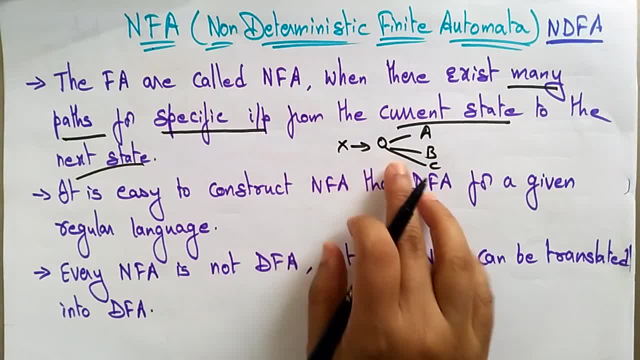 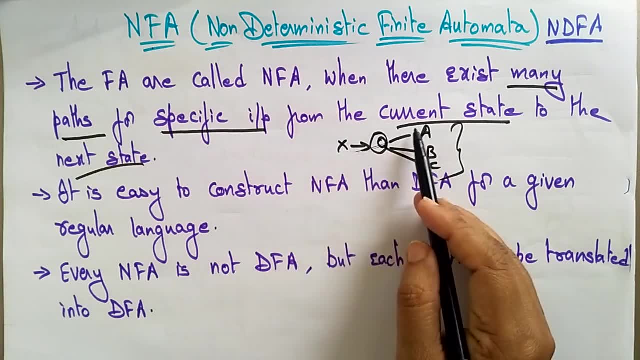 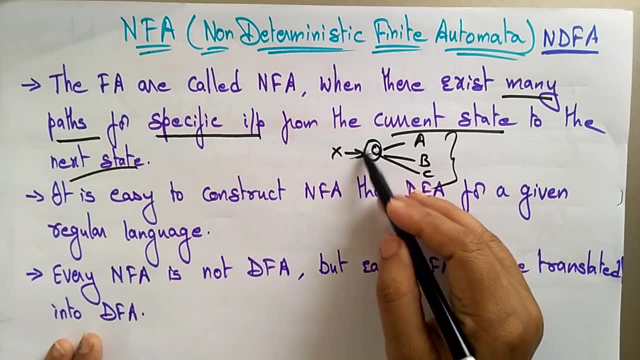 go to the state E, Suppose it is coming from X, the 0 state can. the input can go to any number of states Means so many paths are there. The main difference here, the NFA and DFA, is in the DFA only the specific input can go to the 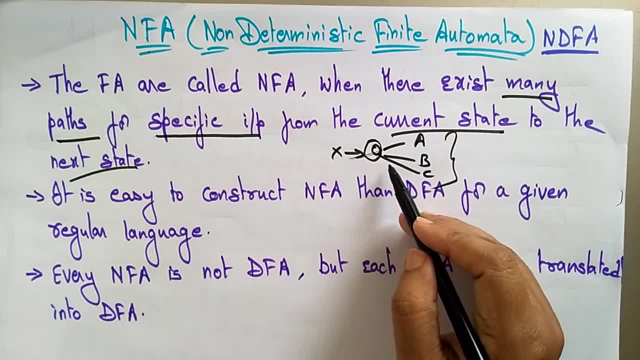 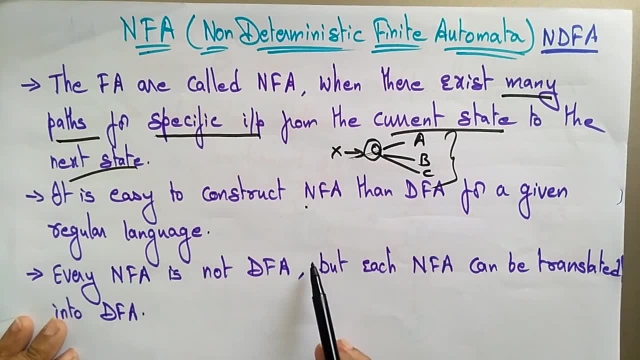 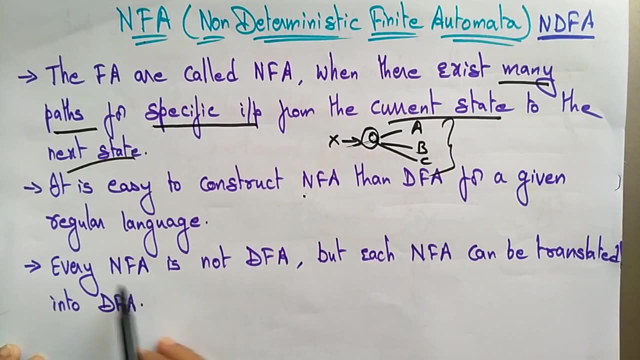 specific only to the one path, But here the many paths can exist for the one specific input And it is easy to construct NFA than DFA. for a given regular language, If any language is given, to construct NFA is very easy when compared to the DFA. Every NFA is not DFA. Remember that. 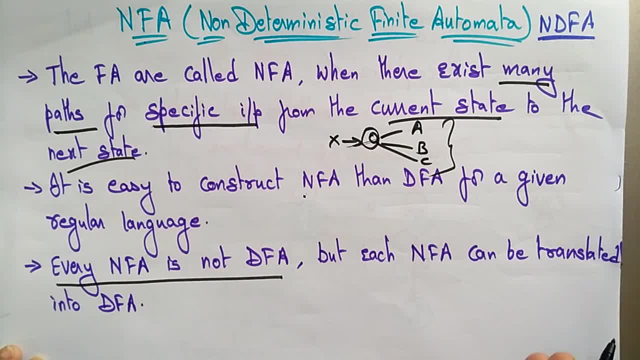 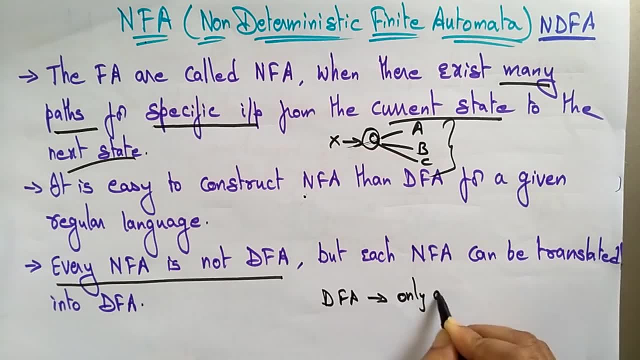 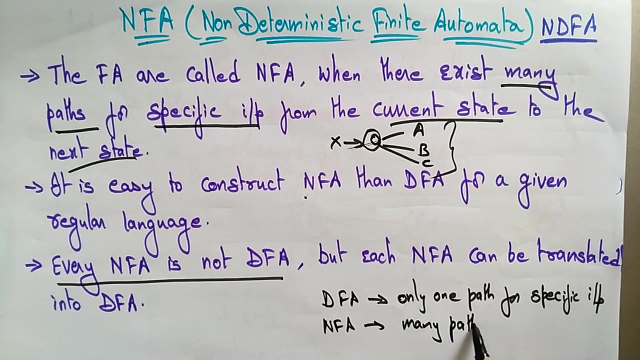 Every NFA is not DFA. Why? Because DFA is having only one path for specific input, Whereas NFA is having many paths for specific input. So every NFA is not DFA because NFA is having multiple paths. Multiple paths are not accepted by the DFA, But each NFA can be translated to DFA. 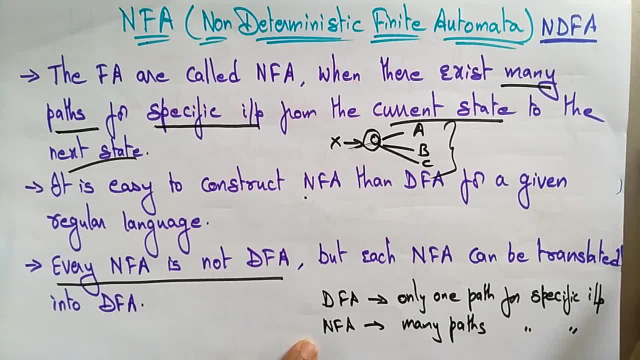 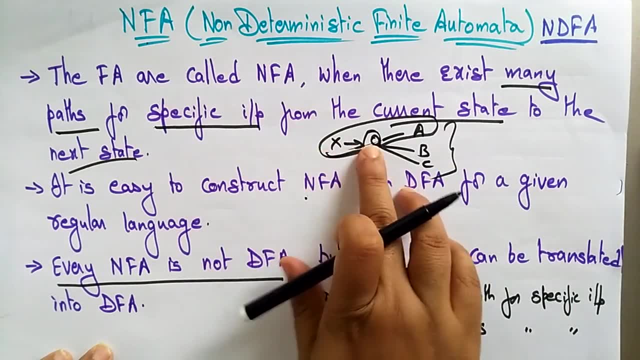 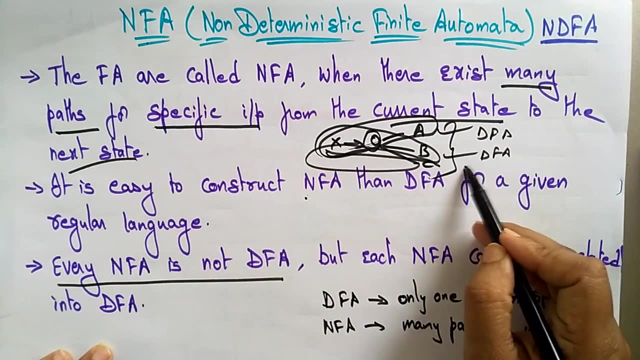 But you can take one path and you can translate that path to DFA. Is it possible? Right? Because you just take this path and construct. this is an NFA. You can take this path and this is DFA. Okay, And you can take this path and this is DFA, And you can take this path. any one path, it is DFA. 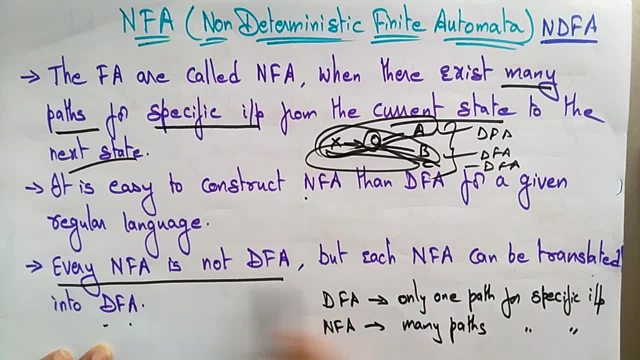 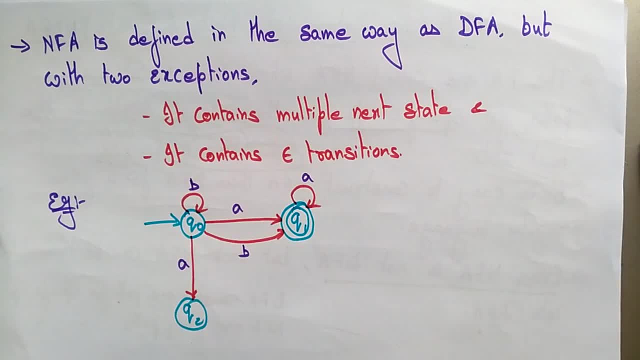 So NFA can be translated to DFA, but every NFA is not DFA. Remember that point. So NFA is defined in the same way as DFA, but with two exceptions. So what are the two exceptions? It contains multiple. next states: 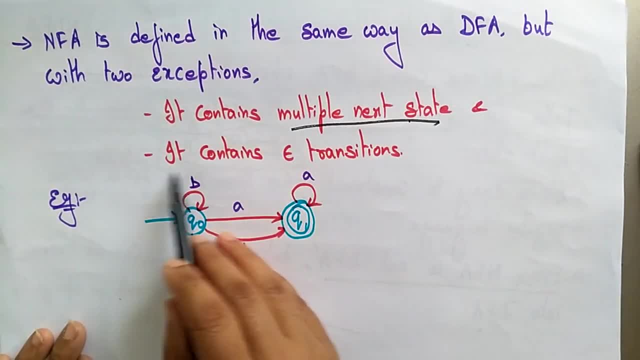 So for each input there are multiple next states are there And it contains epsilon transition. also, In NFA the epsilon transition is possible, Whereas in DFA there are no epsilon transition, So that I will explain in the next video What is this epsilon transition. 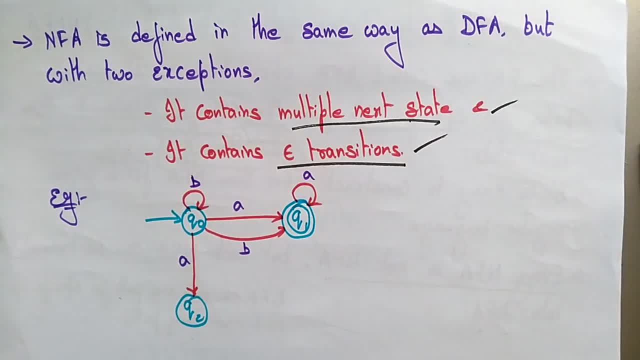 Now let's talk about this multiple states path. I said it contains two exceptions. It contains multiple next states. So here you can see this is an NFA. How can I say this is NFA? Because here the same input, specific input, has multiple paths. 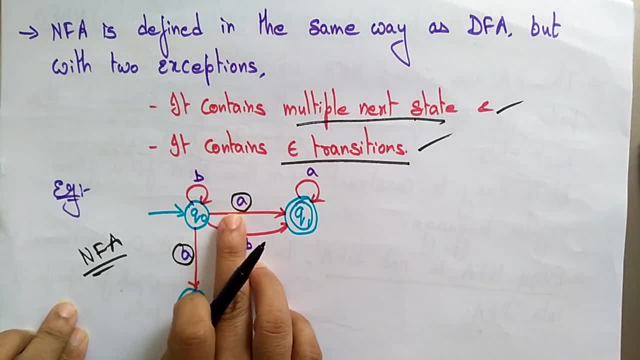 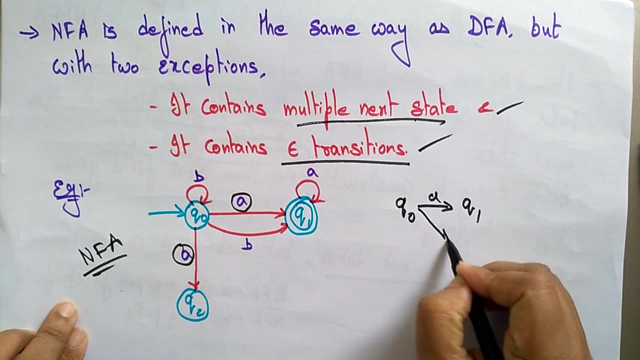 How So here Q0 on A. Q0 on A goes to Q1 and Q0 on A goes to Q2. also, Multiple next states are there? Okay, The Q0 on A goes to Q1 as well. It goes to Q2.. 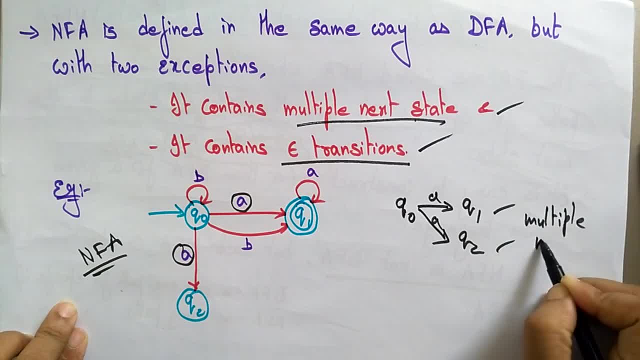 So these are multiple. next states: So whenever you see in the diagram you can easily understand is it DFA or NFA. So DFA, you don't have the multiple states. Okay, Only one symbol can goes to one state only. 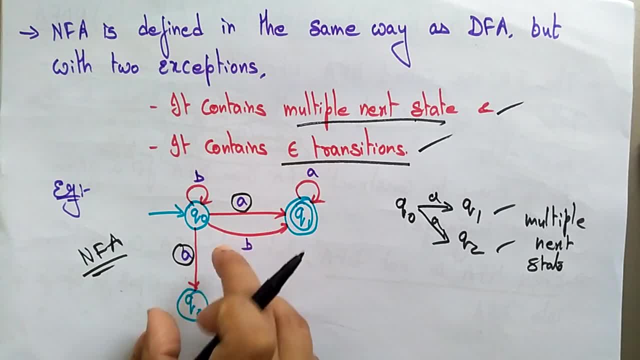 It doesn't goes to the multiple states. The same symbol, specific input, cannot contains the multiple states. Only one state should be there. One specific path should be there in the DFA, But in NFA you can have the multiple states, Okay. 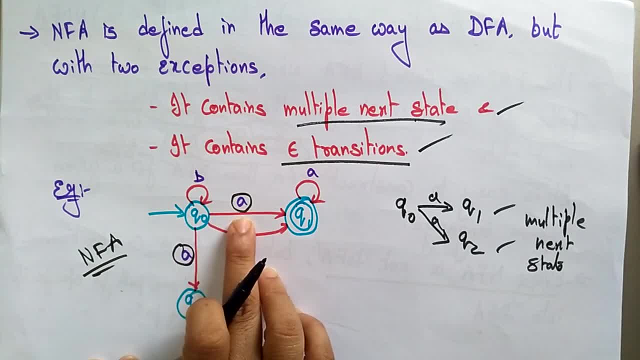 So the Q0 for input A. there are two next states: Q1 and Q2.. Okay, Similarly, the Q0 on B. okay, The Q0 on B goes to the next state, to Q0 as well as to the Q1.. 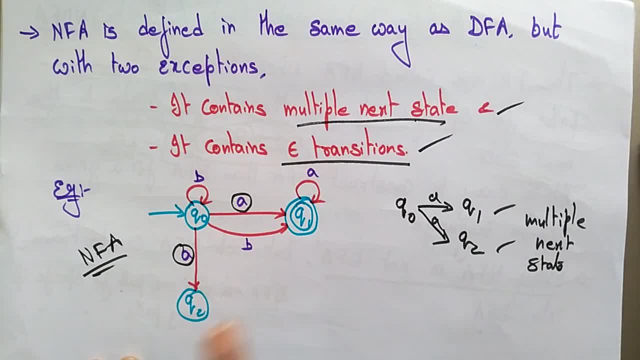 So thus it is not fixed or deterministic, So with a particular input, where to go to the next state. So hence finite automata is called. we call it as a non-deterministic finite automata. Okay, So because it is not fixed, 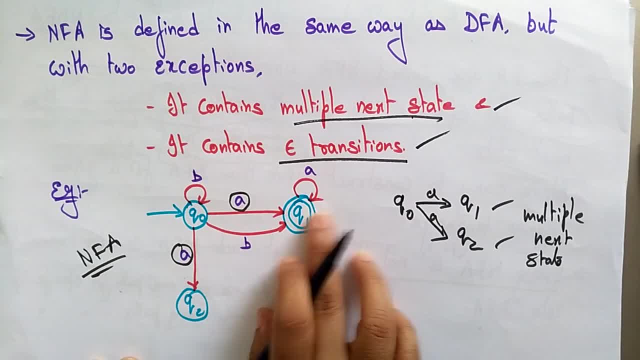 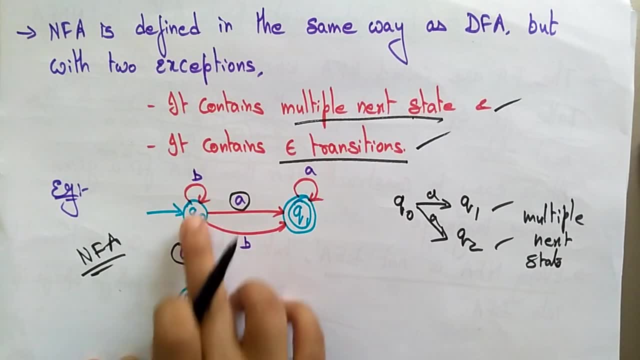 Okay, Specific path is not fixed. There are multiple paths. Suppose this path is not suited, it is not reaching the destination. you can select the another path. Okay, Suppose if first I had taken this path. Q0 on A goes to Q2.. 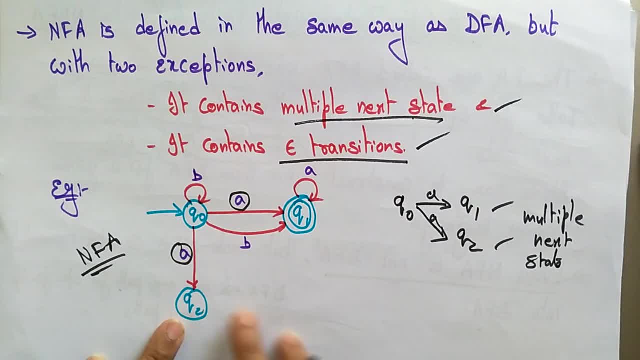 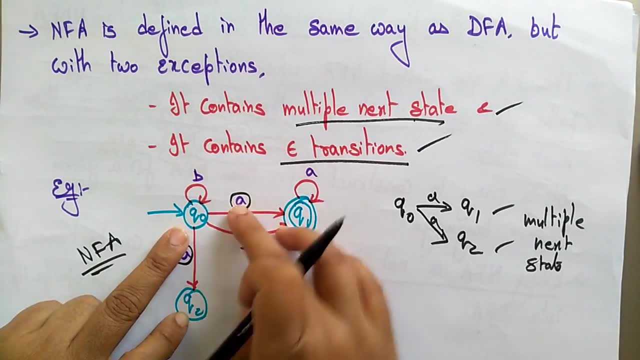 So here from Q2, I am not going to anywhere, I am just moving to the phi epsilon. So I can select this path. Q0 on A goes to Q1, reaching the final state. I will accept this string. 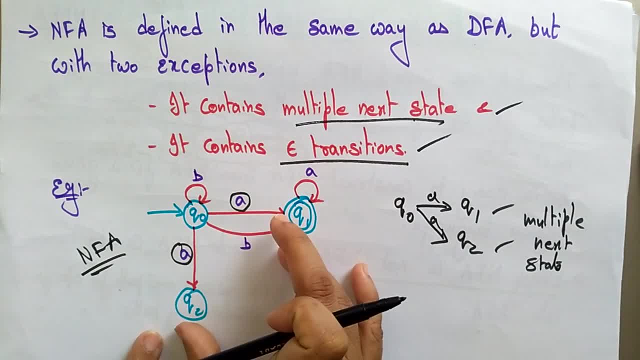 Okay, These are the multiple paths are there. So in that multiple path I can select this string. Okay, In multiple paths, you can select any one of the path. So this is a main advantage of using this NFA. 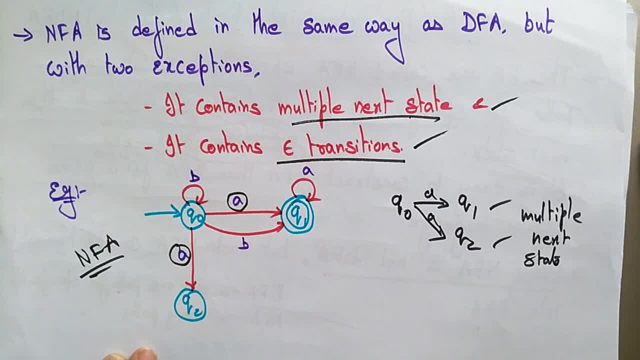 I am having the multiple paths. I can select any path, But in DFA there is no multiple paths. Either you can accept or you can reject. So in this NFA you can take the multiple paths. From that multiple paths, select one of the best path and which is going to be accepted. 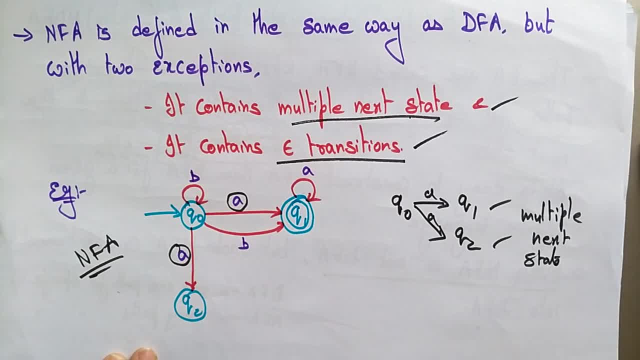 and which is going to reach the final state. That string I can accept, That path I can choose. So that is the main advantage of using NFA. So you will get a doubt why I am going to use NFA if DFA is there. 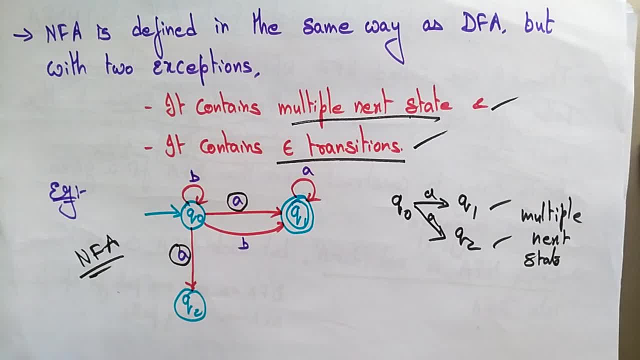 Because DFA is fixed. In some situations the DFA will be used, But in some situations NFA will be used, Because here the backtracking is there And suppose, if you want to move from, if you want to, anyhow, you want to reach to the final. 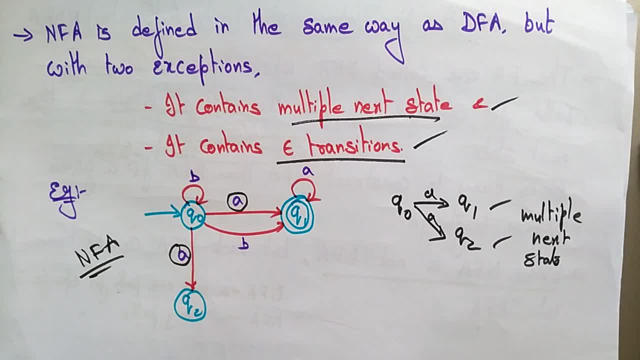 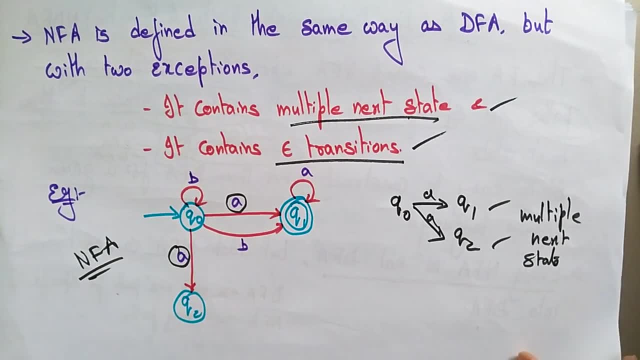 state means you can select the multiple paths. So in some situation there is a way of selecting the multiple paths. In that cases we will use this NFA. So I hope you understand clearly what is the difference between the NFA and DFA. 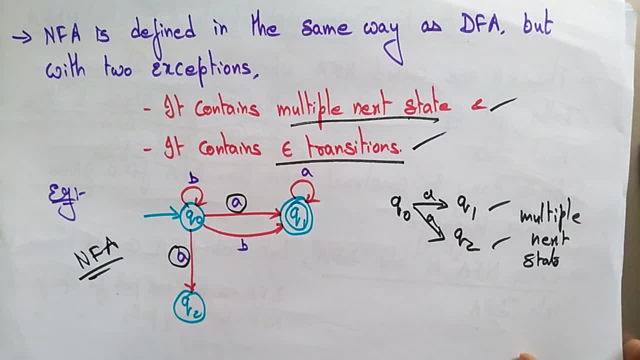 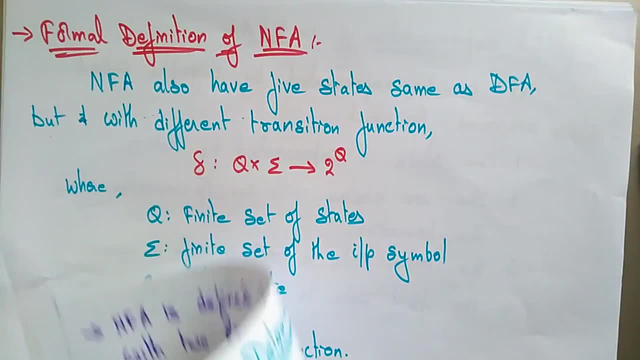 NFA is having only the single path which leads to the next state, Whereas in DFA. whereas in NFA, it contains a multiple next paths. Let's see the formal definition of NFA. NFA also have the five states, same as the DFA. 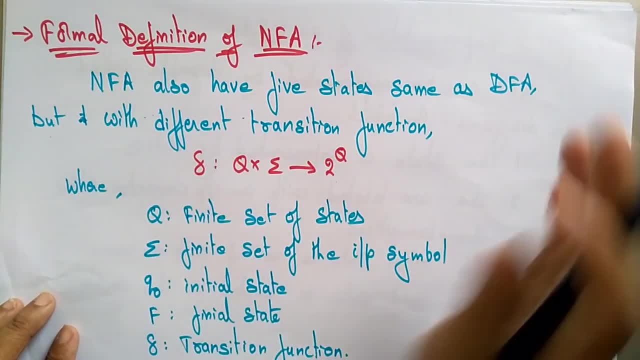 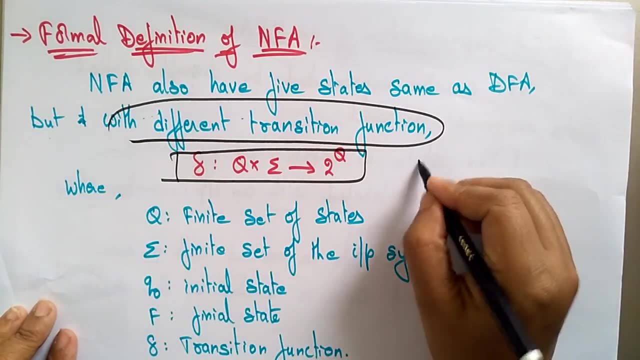 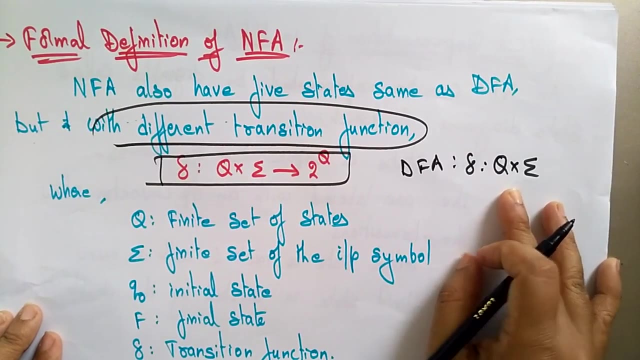 So it is just having the five tuples, just as a DFA, But with the different transition function. So what is the different transition function? This is the transition function, Whereas DFA transition function is: delta is equal to Q into sigma- That is the current state- into input. current state input symbol leads to the next state. 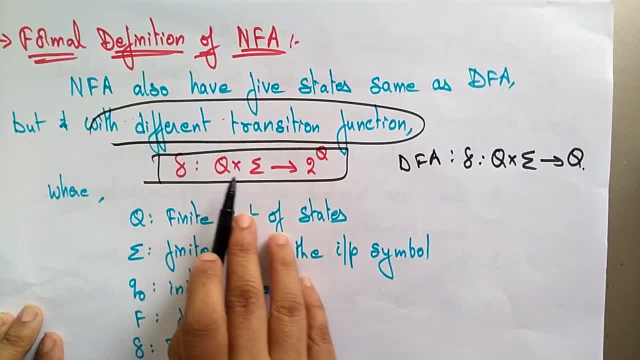 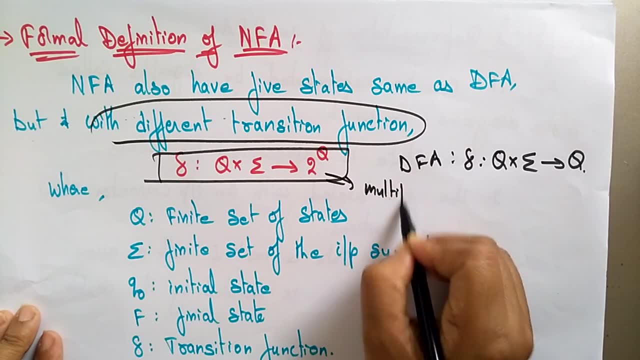 Okay, But here in NFA the current state with input symbol leads to multiple states. So that's why it is 2 power Q, Multiple states. will you will get Multiple states. That is the main difference between the NFA and DFA.